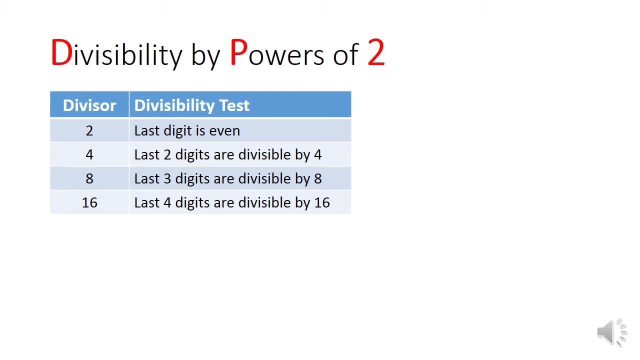 By 8, we only need to check the last 3 digits, and for 16, we check the last 4 digits. and this goes on. The proof isn't that difficult, but let me just show you the divisibility for 4.. I'm going to write out a very long number: AB all the way to XYZ. 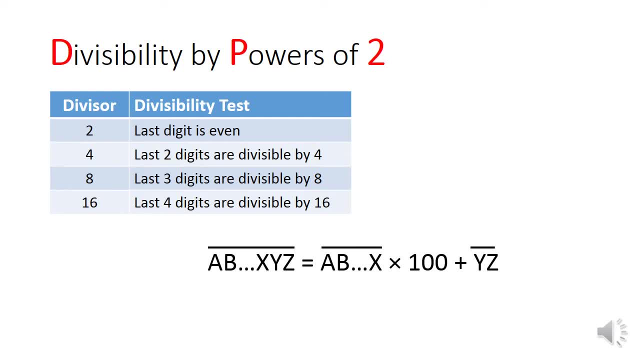 I'm going to write out a very long number AB all the way to XYZ. I'm going to write out a very long number AB all the way to XYZ. I'm going to use an overbar as a symbol for concatenation. 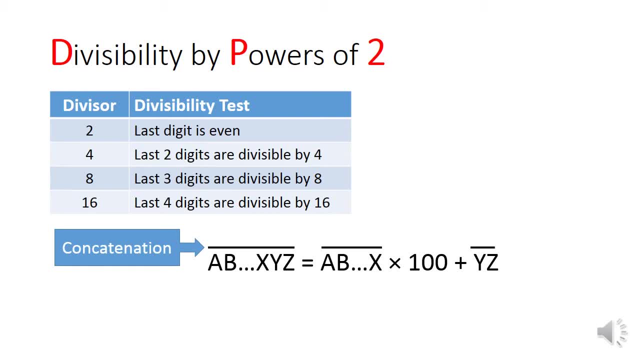 I'm joining these symbols together to form a single number, with each letter representing a digit within that number. This is to prevent misinterpreting this as A multiplied by B, multiplied by C, all the way to Z. Next, I can write this number as a string of AB all the way to X, multiplied by 100. 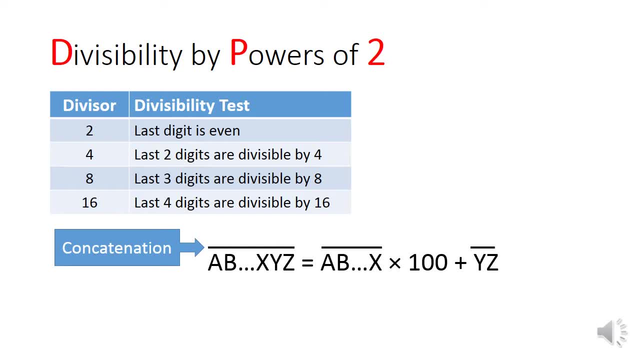 Next, I can write this number as a string of AB all the way to X multiplied by 100, plus the concatenation of Y and Z. I can see that because 100 is divisible by 4, the first group highlighted in red must be divisible by 4. 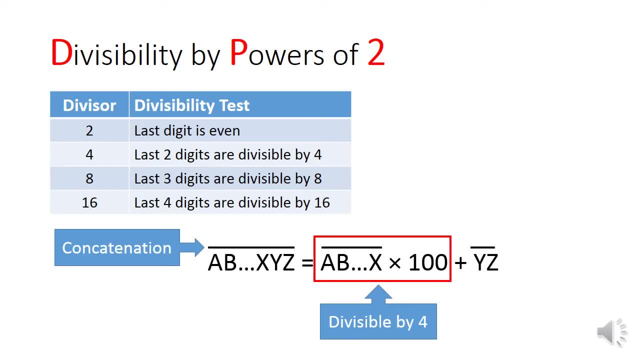 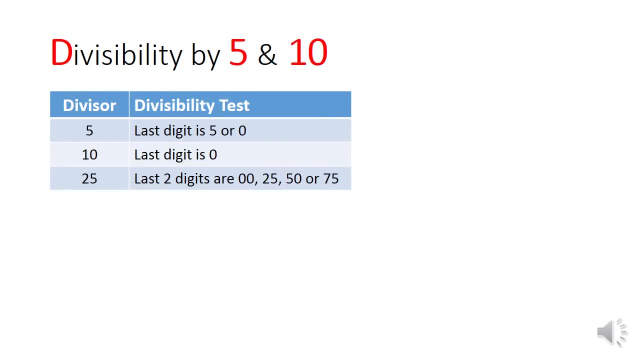 Hence to check the divisibility by 4, I only need to check the divisibility of the last 2 digits. For divisibility by five or ten, checking the last digit will do Anything with. the last digit of B is divisible only by four digits. 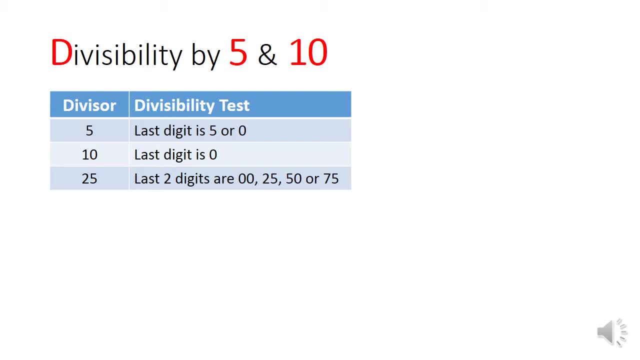 digit of 5 or 0 is divisible by 5, and only a last digit of 0 will be divisible by 10.. The divisibility test for 3 and 9 requires you to sum up the digits and check if that sum is divisible by 3 or by 9.. The logic behind this test is that if I express the concatenated 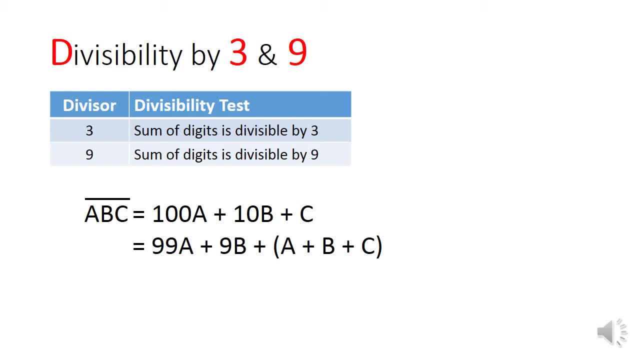 number as an algebraic expression like a 3-digit number, ABC. ABC is actually 100A plus 10B plus C. The trick is then to split the 100A into 99A plus A and the 10B into 9B plus. 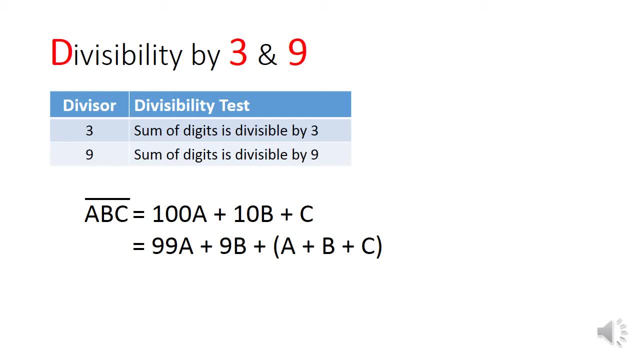 B. You then regroup the expression into two parts: 99A with 9B as one group. you can see that this part of the expression is clearly divisible by 3 or by 9.. Hence we only need to check the second group, A plus B plus C, which is the sum of the digits. 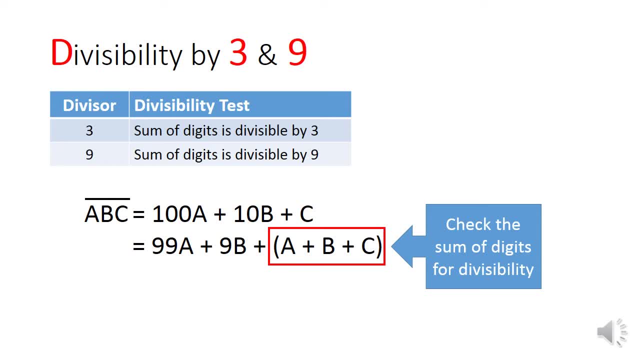 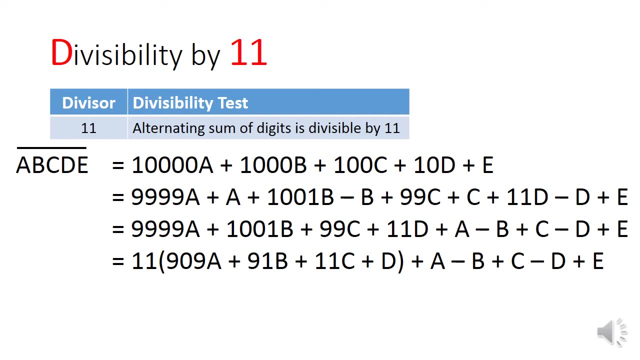 and to see if that is divisible by 3 or by 9.. If the sum is divisible by 3, the entire expression would also be divisible by 3.. And the same goes true for 9.. For the divisibility test of 11, I apply an alternating sum of digits. This means to take: 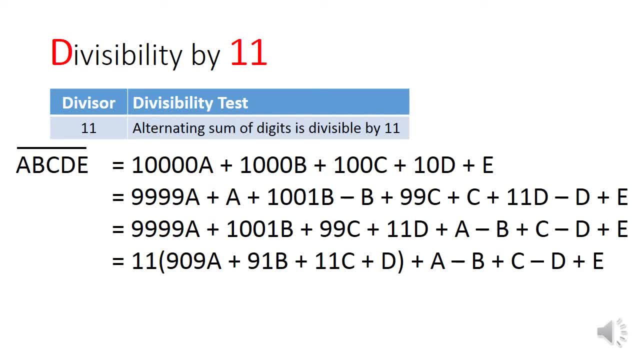 its first digit and the second digit and the third digit and the fourth digit and the fifth digit and the sixth digit and the seventh digit and the eighth digit and the seventh digit. subtract the second digit, add the third digit and keep alternating. 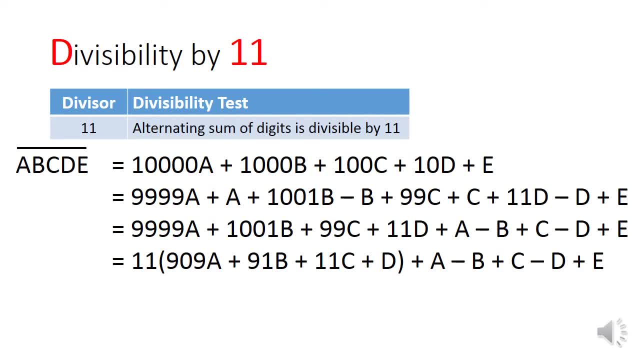 between adding and subtracting till you reach the end of the number. You then check the divisibility of that particular alternating sum by 11.. The proof is presented here By taking a 5-digit number such as ABCDE and expressing it as 100A plus 1000B plus 100C. 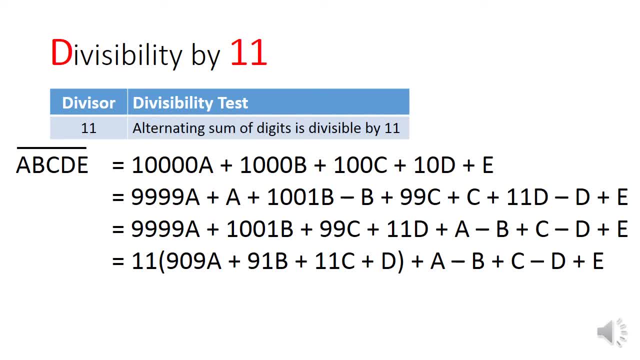 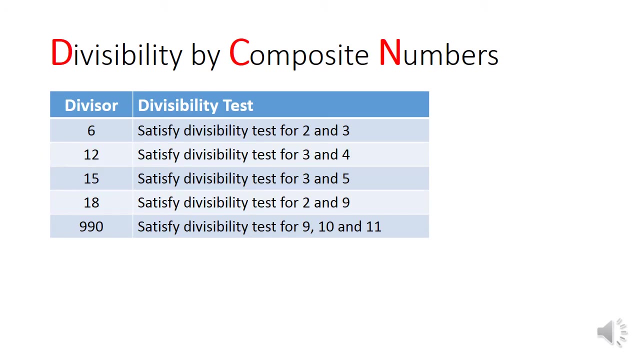 plus D. I can manipulate this algebraic expression into two groups. The first group is 11 times of 909A plus 91B, plus 11C plus D. This is clearly divisible by 11.. Hence I only need to check the second group, which is the alternating sum For the divisibility of composite numbers. 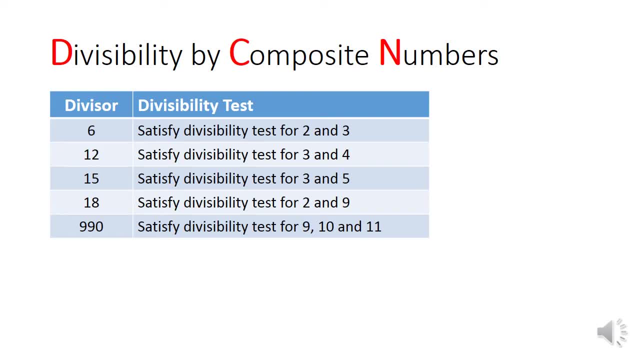 you have to conduct separate divisibility tests For the divisibility of composite numbers. you have to conduct separate divisibility tests For the divisibility of composite numbers. you have to conduct separate divisibility tests, For example, to test for divisibility. 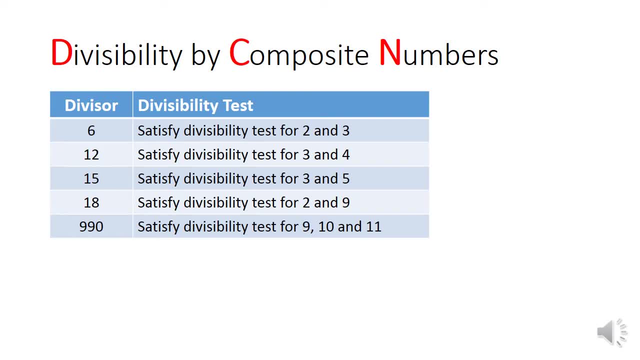 by 18, you check for divisibility by 2 and then check for divisibility by 9.. You have to be careful that the lowest common multiple of each test have to equate to the divisor of the test you are trying to implement. 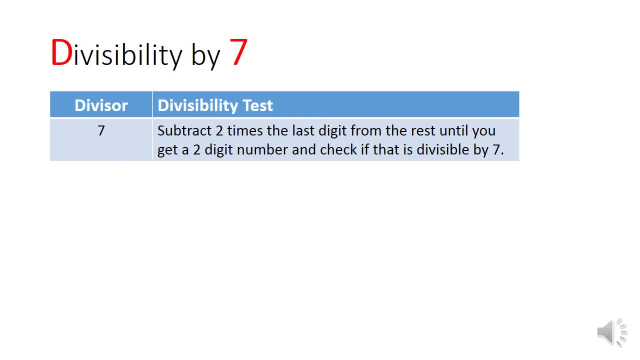 Normally this test would be sufficient, but let me also cover the test for you to see the difference for weirder prime numbers such as 7 and 13.. Hopefully, by walking you through the test and the logic behind these tests, you can create your own tests for other prime numbers. 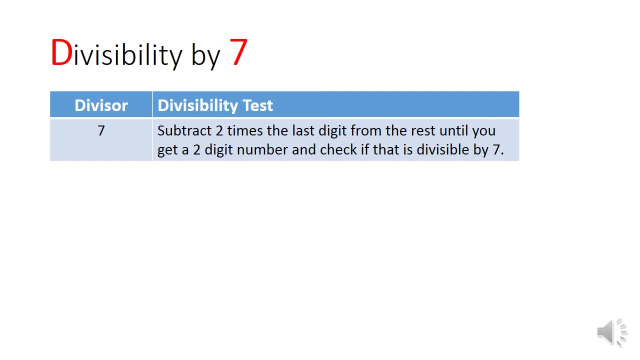 For 7,. the test is to subtract two times the last digit from the rest of the numbers until you can find a number small enough that you can check for divisibility by 7, usually a one to two digit number. Let's take an example. 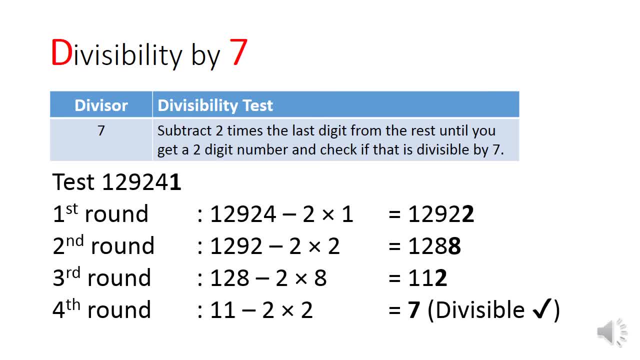 The number 129,241.. We first take the first five numbers- one, two, nine, two, four, and subtract two times of the last digit: one, You get one, two, nine, two, two. Then you take one, two, nine, two. 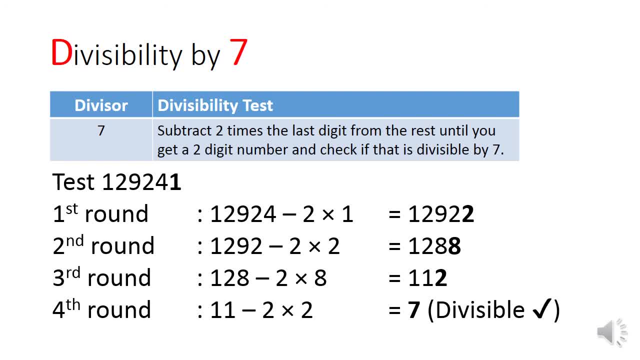 and minus two times the last digit two, and you get one, two, eight, eight. Then you take one, two eight minus two times the last digit eight, you get one, one, two. You can do this one more time. 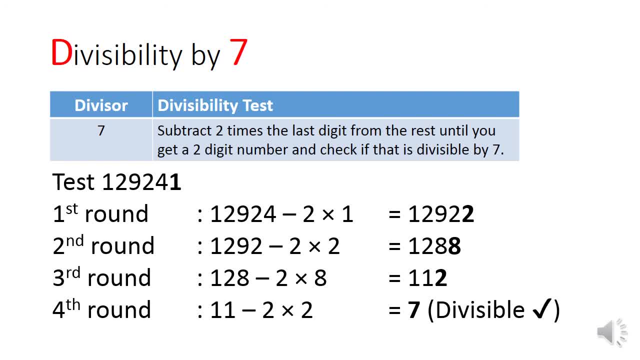 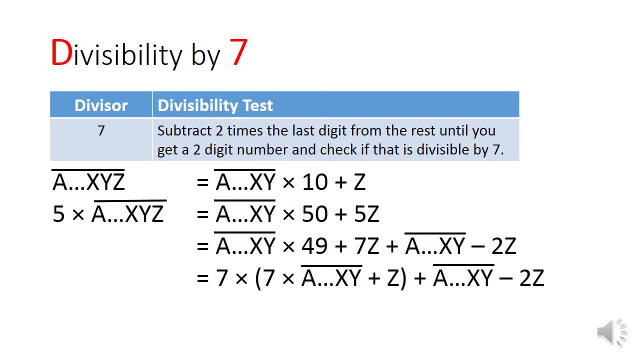 and you'll get seven, two, nine, two, seven, which is obviously divisible by seven. So one, two, nine, two, four, one will also be divisible by seven. Let's look at how this test work. First, I separate the last digit, z, from the rest. 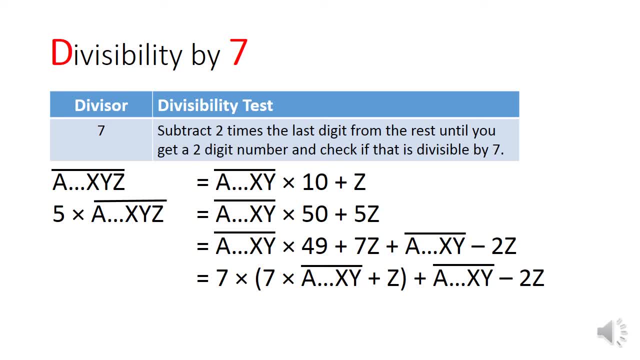 This gives me the concatenated number a to xy, multiplied by 10 plus z. Next I multiply both sides by five. Two points to note here. First, because five and seven are divisible, seven are co-prime, meaning that they have no common factors. 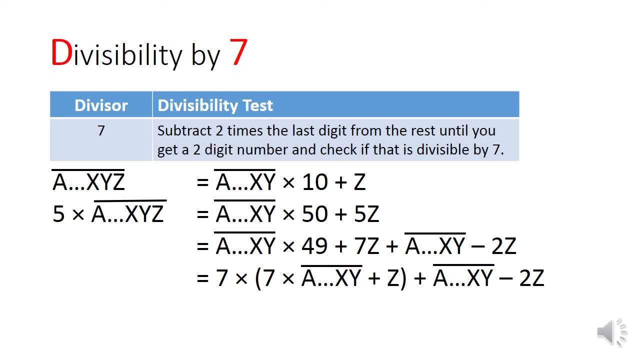 If five times the original number is divisible by seven, the original number must also be divisible by seven. Second, I'm doing this because 50 is just one more than 49, which happens to be a multiple of seven. This allows me to rearrange the expression into two groups. 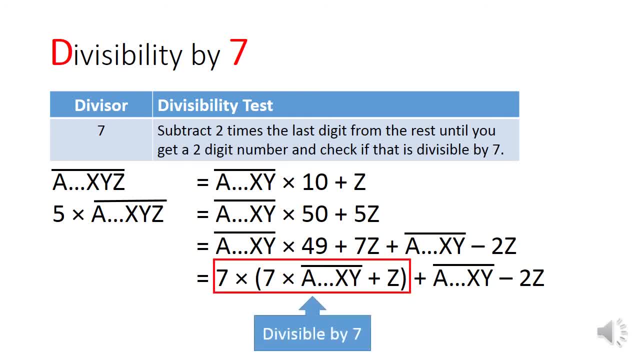 The first group, highlighted in red, is clearly divisible by seven. The second group is the portion that I need to check for divisibility, And if that number is large, we can perform this trick over and over again. The caveat here is that any non-zero remainder. 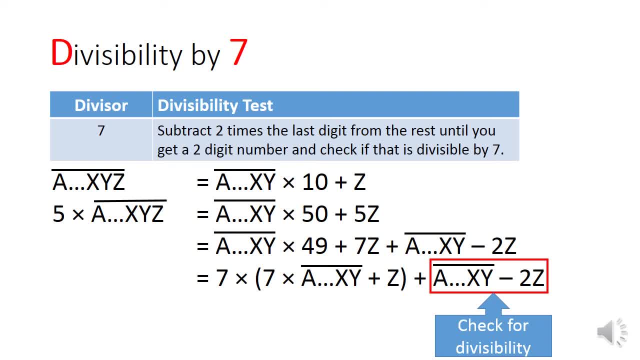 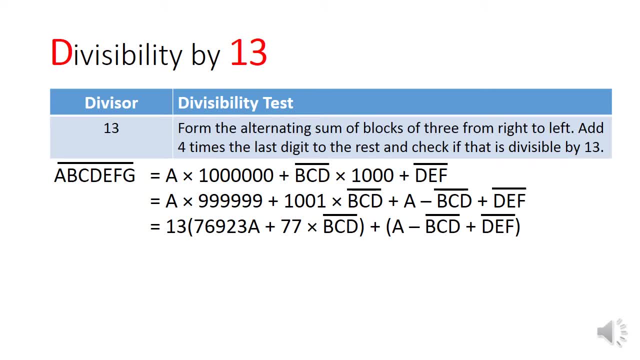 that you get from this test will not be the remainder for the actual division For 13,. we can first do an alternating sum of blocks of three digits from right to left. Next we can add four times the last digit, z last digit, to the rest to check if that is divisible by 13.. Let's have a look at. 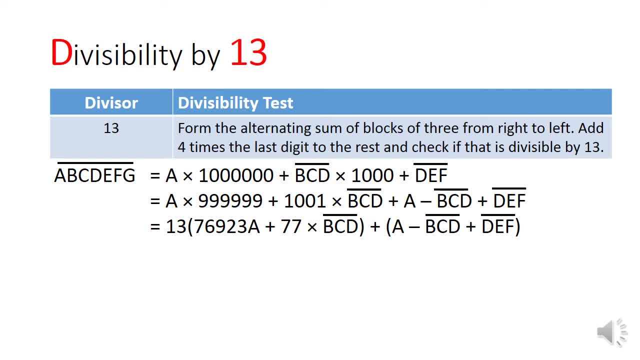 a proof for a seven digit number which is easily extendable to larger numbers. You can see that the letter A is in the millionth place, so it's A times 1 million. This is 1 more than 999,999, which turns out to be a multiple of 13.. 13 times 76,923.. 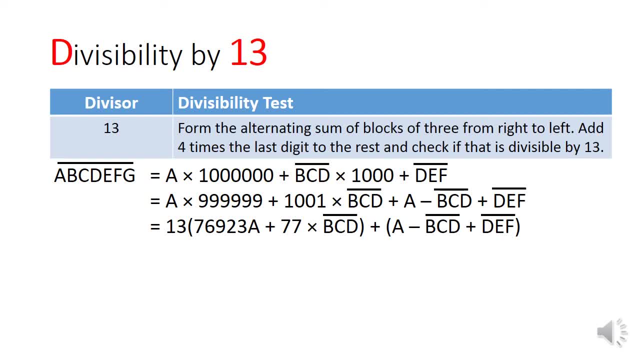 The chunk of three digits BCD are in the thousandth place. That turns out to be 1 less than 1001, which is also a multiple of 13.. 13 times 77. This allows one to re-express the number into: 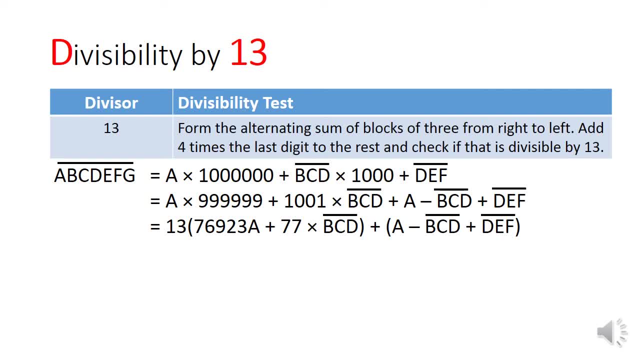 two chunks. The first part is a multiple of 13 and the second chunk, which I've highlighted in red, is the alternating sum of blocks of three digits which needs to be checked for divisibility Subtitles by the Amaraorg community. For a three digit number, like ABC, we can express this as A times 100 plus B, times 10 plus C. 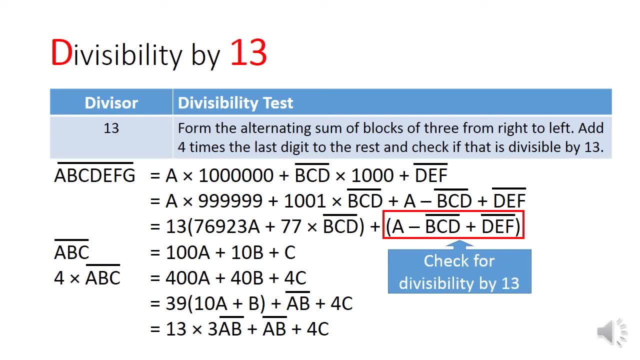 Next, you multiply both sides by 4.. The rationale is the same as before: 4 and 13 are co-prime, And if 4 times the original number is divisible by 13,, the original number would also be divisible by 13.. You also want 40, because this is 1 more than 39.. 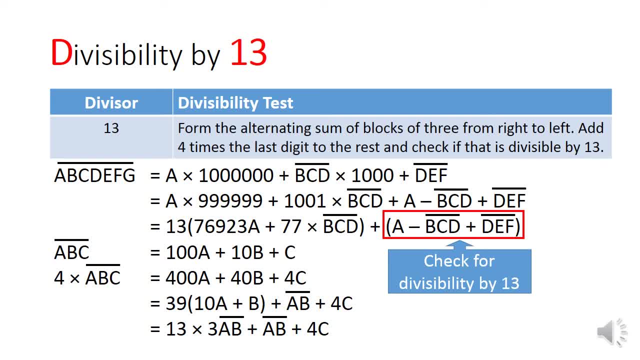 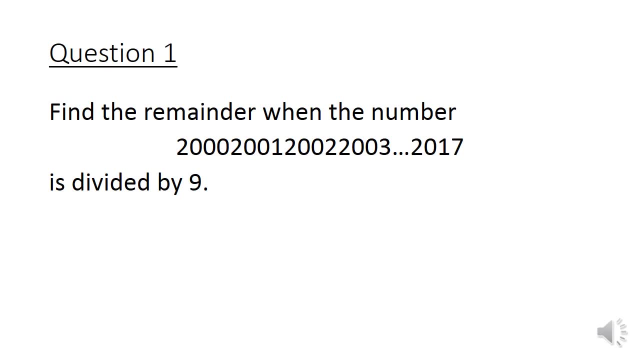 You're very well prepared. You recognize that the 짜는 fights for a number that is divisible by 385, and that the Cena is not divisible by AL Eine when her number is divisible by 40.. 2 times 0. It means it is divisible by 1 times 30.. 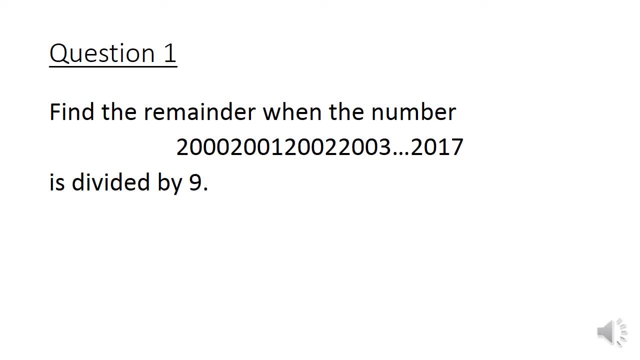 Er欠 array: 2 times 1 equals to 2, meaning it is divisible: 2, 2, 0, 0, 3, all the way until 2, 0, 1, 7,. find the remainder when that number is divided. 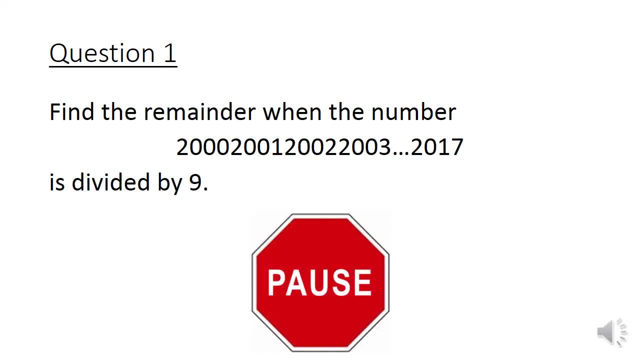 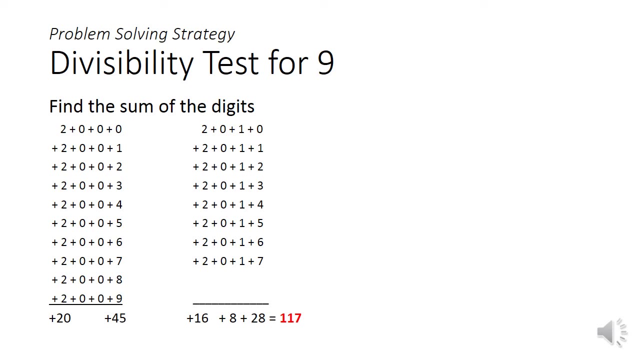 by 9.. I'm going to ask you to pause the video here to try this question. Recall the divisibility test for 9.. We need to find the sum of all the digits. Using brute force, you'll get 117.. So is 117 divisible by 9? Let's do another sum of digits. 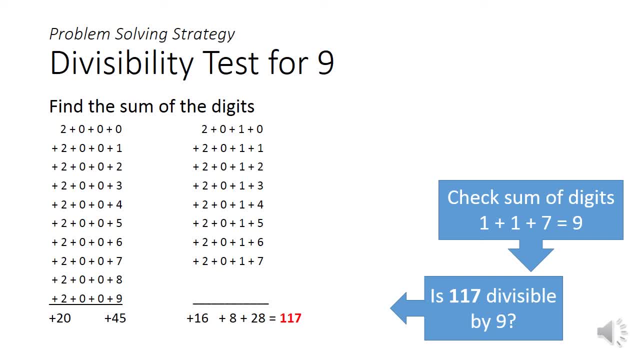 and that will give you 9,, which is clearly divisible by 9.. Hence, 117 is divisible by 9, and a huge number will also be divisible by 9.. Since it is perfectly divisible, the remainder has to be 0.. 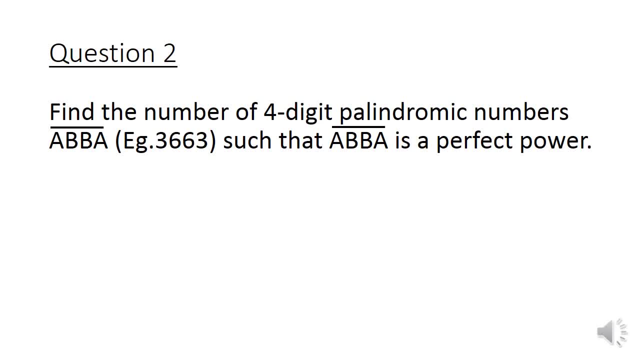 Next question: Could you find the number of 4-digit palindromes that are also perfect powers? Palindromic numbers are numbers that come in the form ABBA. Let me give you some examples: 3663, 7887,. these are numbers which are palindromic When the numbers are read. 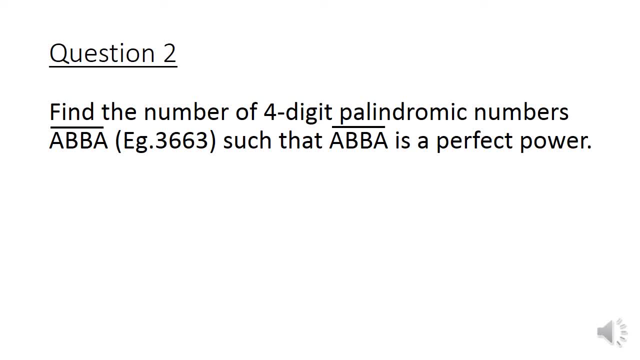 from left to right or right to left, they are exactly the same. The language equivalent of palindromic words are words like noon N-O-O-N, madam M-A-D-A-M, or race car R-A-C-E-C-A-R. Perfect powers are numbers that can be expressed as A to the power. 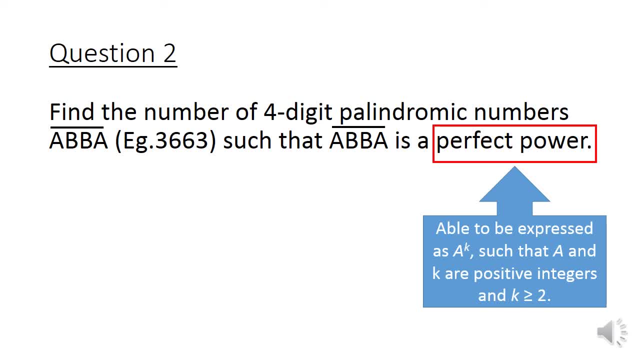 of K such that A and K are positive integers. K has to be at least 2.. For example, 32 is a perfect power. 32 is 2 to the power of 5.. 81,- 81 is 9 to the power. 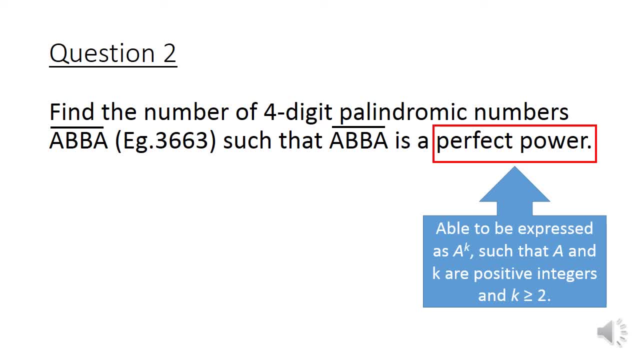 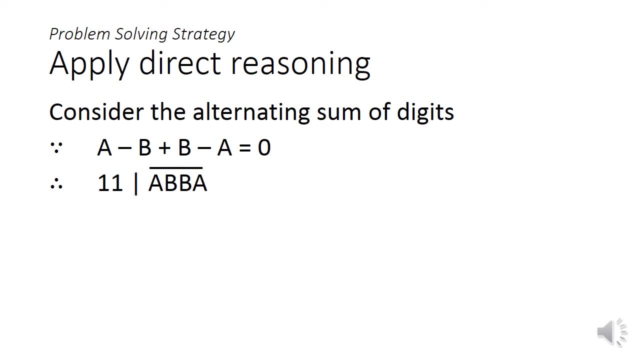 of 2, or 3 to the power of 4.. I am going to ask you to pause the video here to give this question a good try. Let's look at the solution. Let's look at the solution. Let's look at the solution. 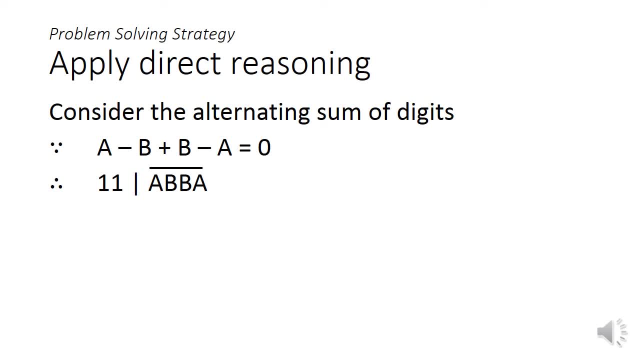 alternating sum of digits a minus b, plus b minus a, we will get a sum of zero. From our divisibility rules we can conclude that 11 divides the four-digit palindromic number a, b, b, a. I would. 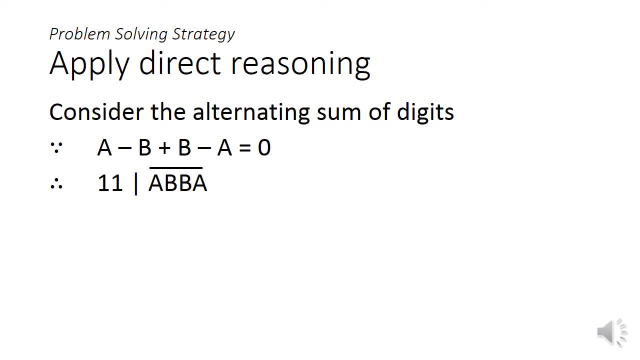 also like to add some comments on the symbols I'm using here. The three dots I'm using represent because, and therefore The vertical line represents divides, that means to divide a number with no remainder, Because a minus b plus b minus a equals zero. therefore, 11 divides a, b, b, a. 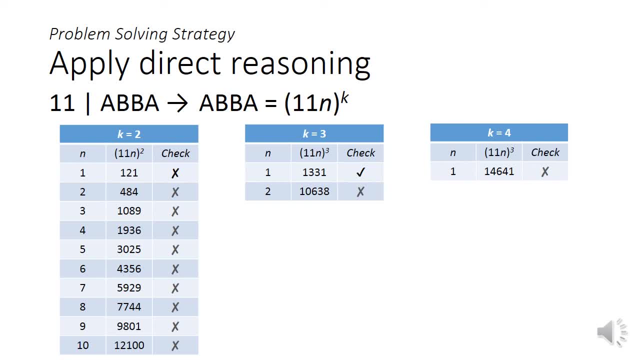 We can then make a list of every perfect power with a base that is a multiple of 11, starting with squares, you can see that 11 square and 22 squares are palindromic, but there are only three digits: 33 square to 99 square are all non-palindromic. Looking at the cubes, 11 to the power of three. 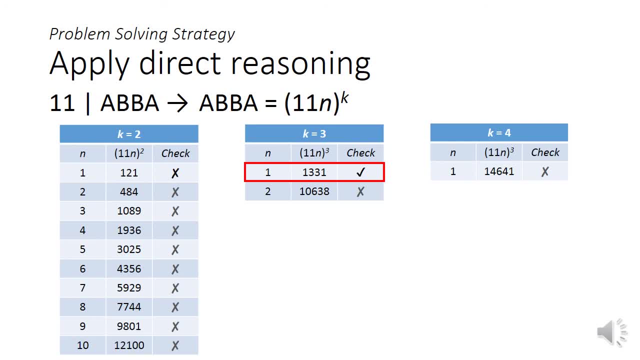 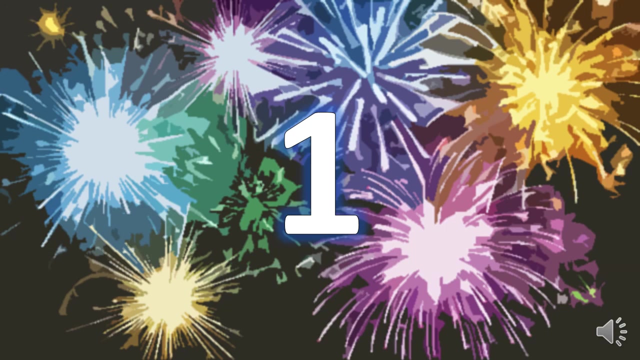 meets the requirement. 22 to the power of three is five digits, so it is too big For higher powers. 11 to the power of four is already five digits, so there is no need to consider any larger power or base. Hence there is only one 4-digit palindromic number. that is also a perfect power. 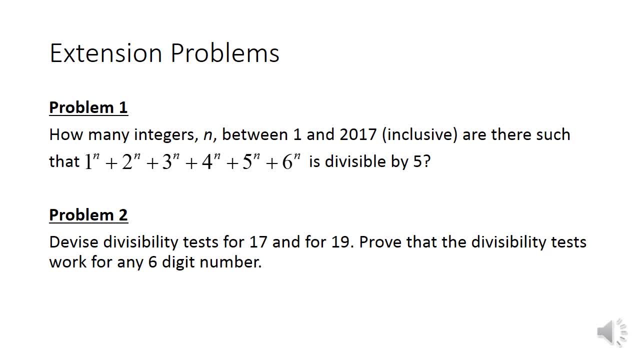 Here are today's extension problems. Problem 1. How many integers n between 1 and 2017 inclusive are there such that 1 to the power n plus 2 to the power n plus 3 to the power n plus 4 to the power n plus 5 to the power n plus 6 to the power n is divisible by 5?? 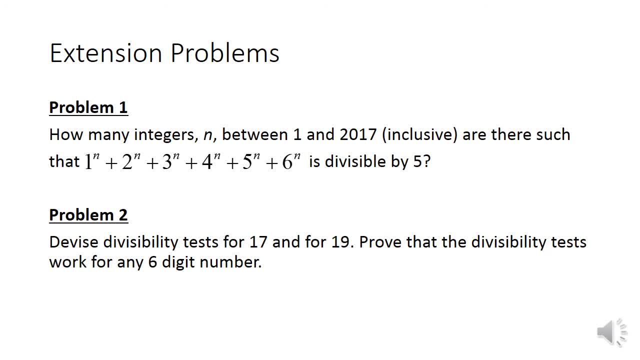 Problem 2. Device divisibility test for the numbers 17 and 19.. Prove that this divisibility test works for a 6-digit number. Solutions to lecture 2's problems have been updated into the info section of the previous video. 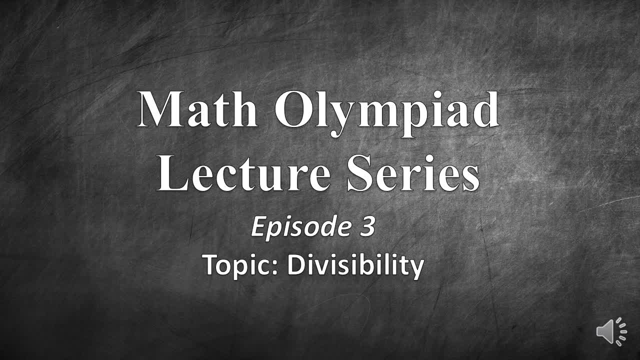 We have come to the end of the third episode on divisibility. Stay tuned to the next episode that will cover the topic of square numbers. Thank you, and have a good day of learning.